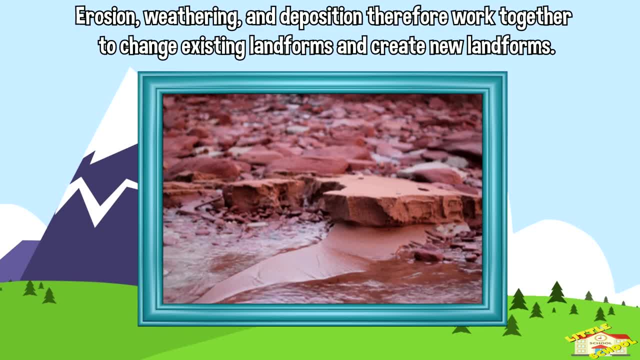 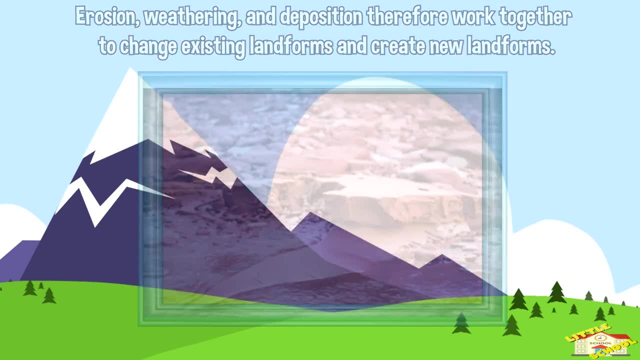 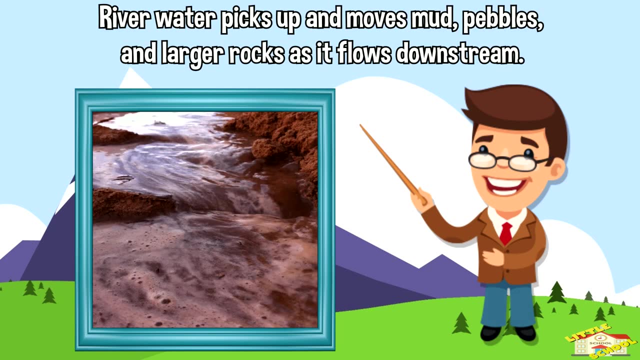 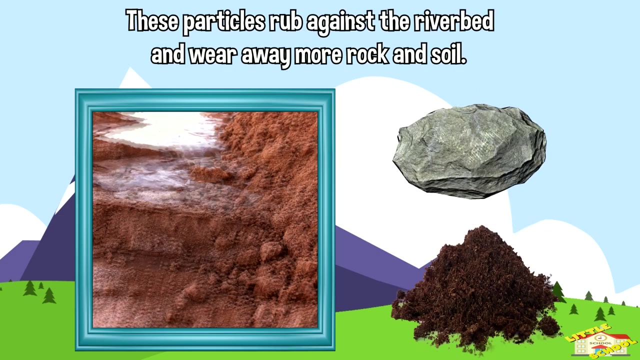 results of deposition. Erosion, weathering and deposition therefore work together to change existing landforms and create new landforms. Let's go over the types of erosion. River water moves mud, pebbles and larger rocks. as it flows downstream, These particles rub against the riverbed. 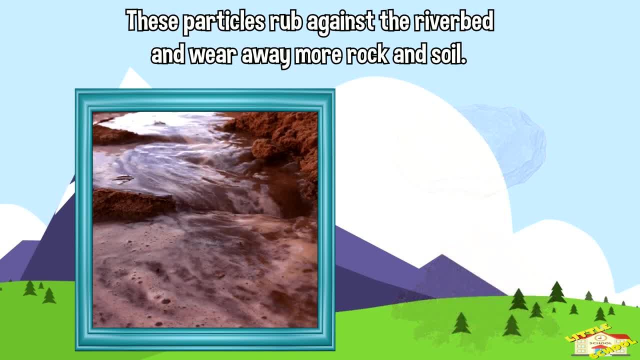 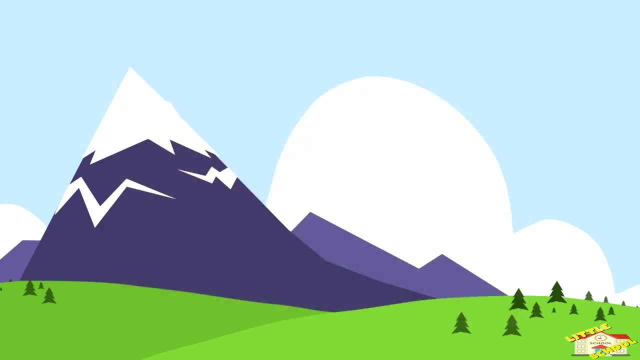 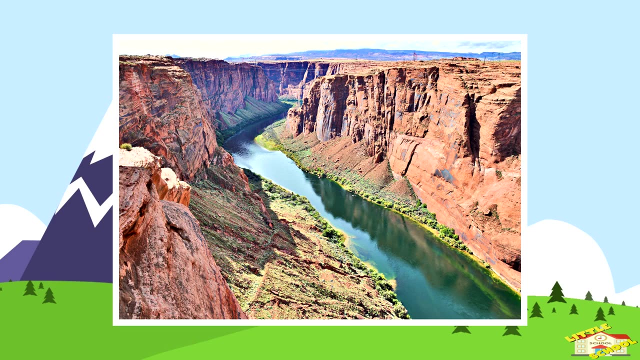 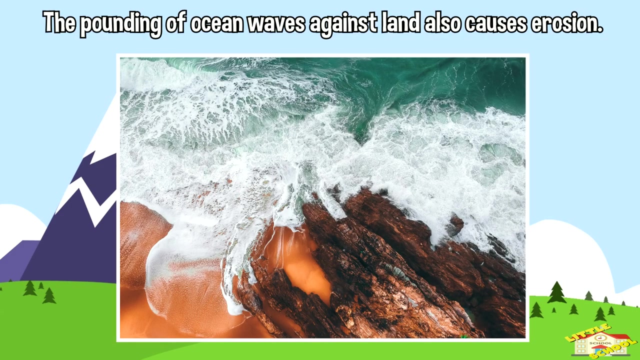 and wear away more rock and soil. This kind of erosion helped to carve the Grand Canyon in the southwestern United States Over millions of years. the swiftly moving waters of the Colorado River carried away bits of earth and rock from the land. The ocean waves against land also cause erosion. The waves constantly move pebbles and sand on. 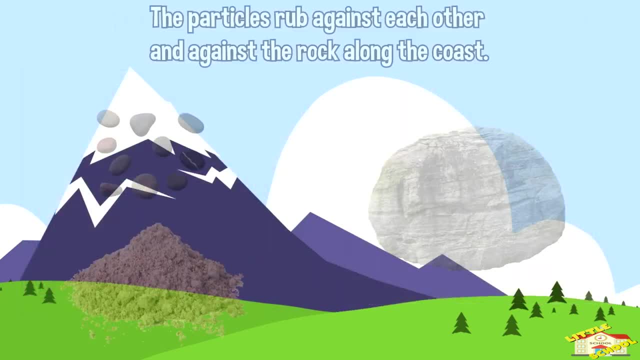 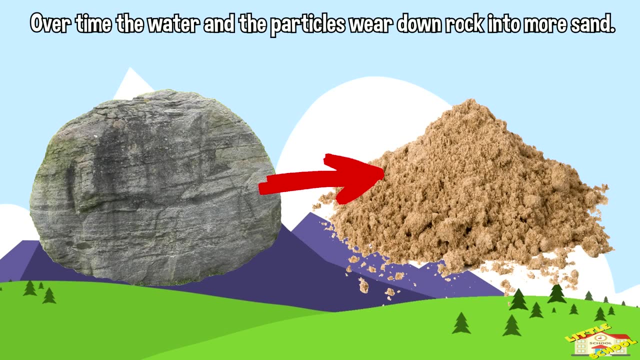 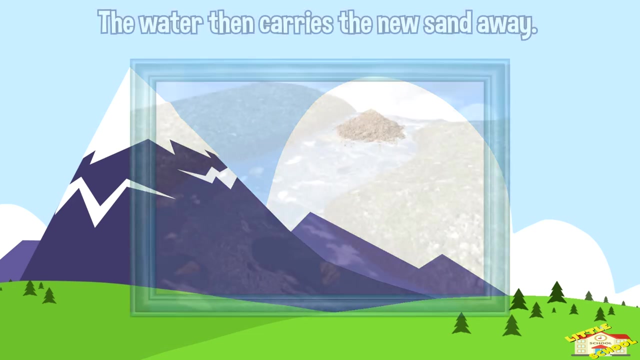 beaches. The particles rub against each other and against the rock along the coast. Over time, the water and the particles wear down rock into more sand. The water then carries the new sand away. Over time, the water and the particles wear down rock into more sand. The water then carries the new sand away. 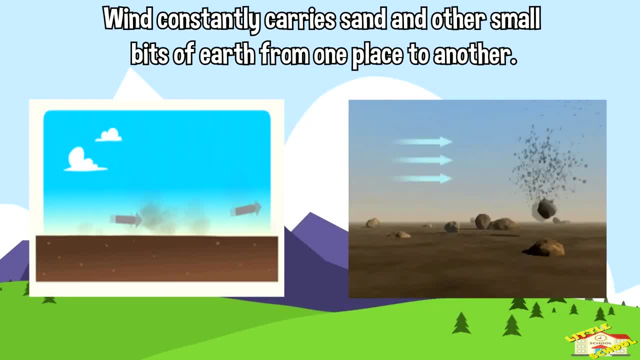 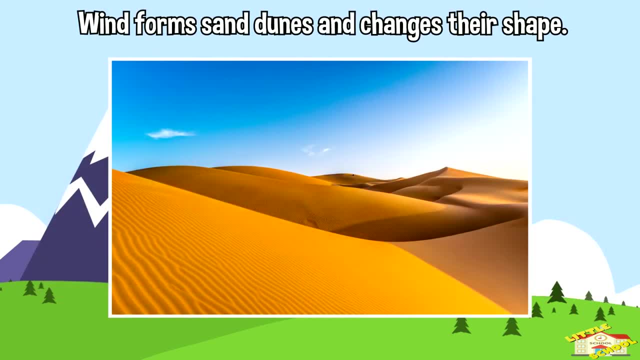 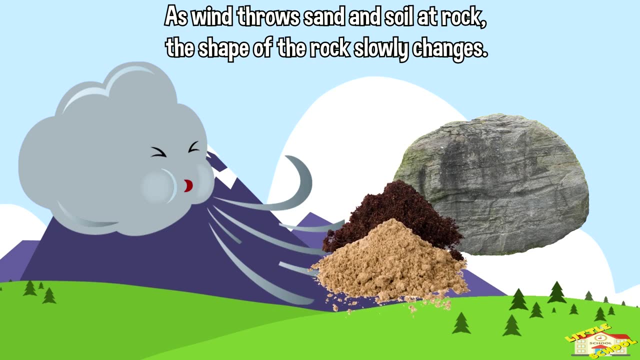 Like waves, wind constantly carries sand and other small bits of earth from one place to another. Like waves, wind constantly carries sand and other small bits of earth from one place to another. Wind forms sand dunes and changes their shape. As wind throws sand and soil at rock, the shape of the rock slowly changes. 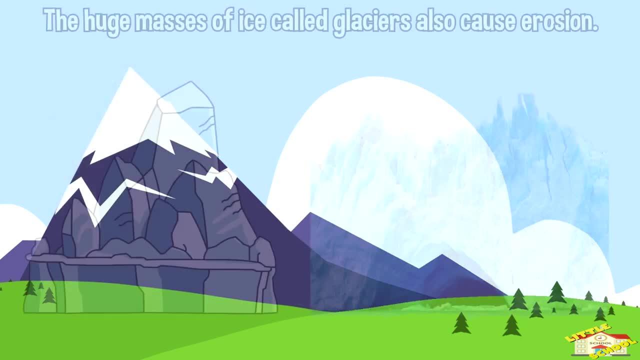 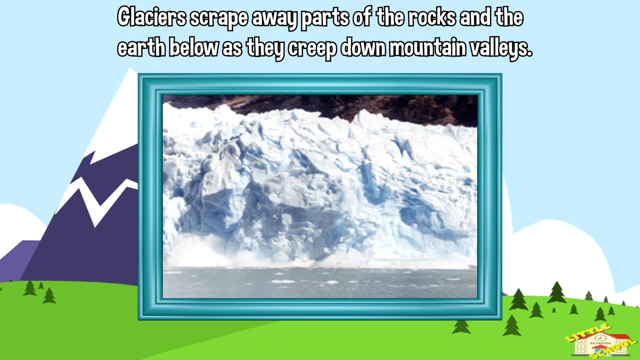 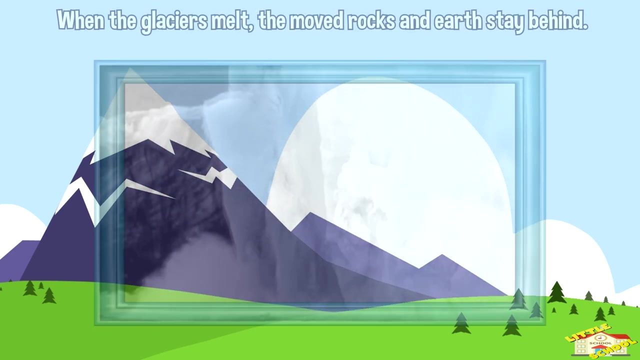 The huge masses of ice-cold glaciers also cause erosion. The huge masses of ice-cold glaciers also cause erosion. Glaciers scrape away parts of the rock and the earth below as they creep down mountain valleys. Glaciers scrape away parts of the rock and the earth below as they creep down mountain valleys. 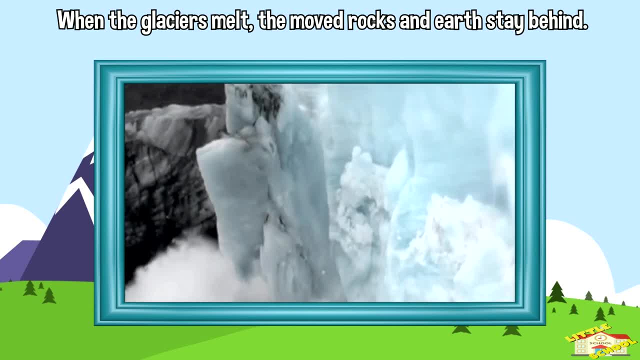 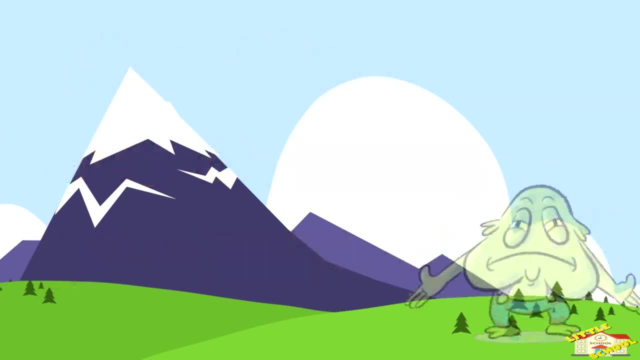 When the glaciers melt, the moved rocks and earth stay behind. Are there any dangers to erosion? Erosion can be very harmful to farmland. Crops depend on rich soil for healthy growth. Crops depend on rich soil for healthy growth. 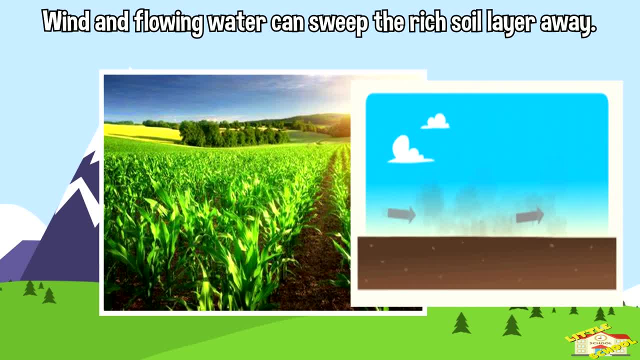 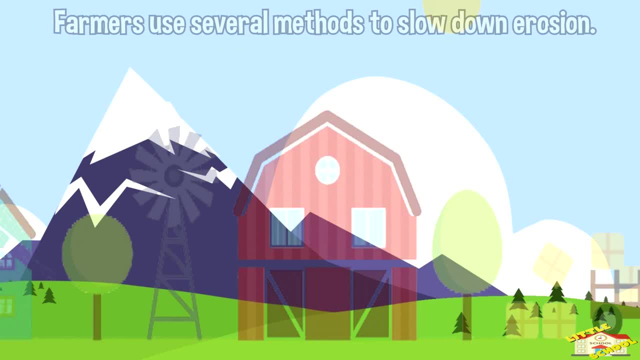 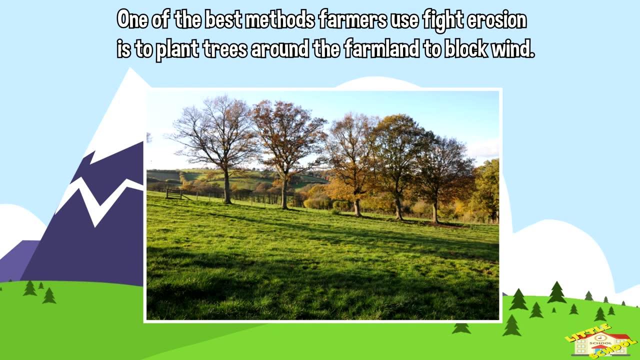 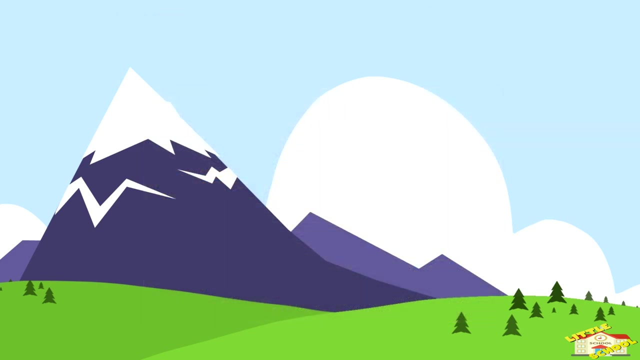 Wind and flowing water can sweep the rich soil layer away. Farmers use several methods to slow down erosion. One of the best methods farmers use to fight erosion is to plant trees around the farmland to block wind. And that is all for today's video. 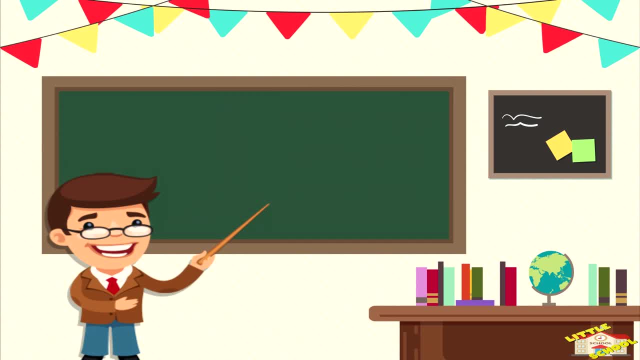 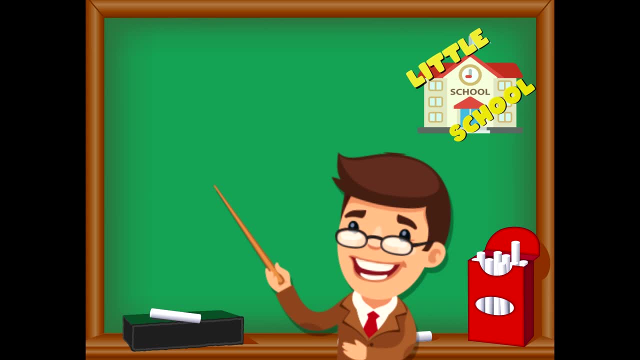 I hope you enjoyed learning about erosion today. Take care now, Bye-bye. If you enjoyed the video and want to see more videos from us, please click the subscribe button. Also give us a like. That will help us. We thank you so much and we do hope that you enjoy our videos. See you soon. 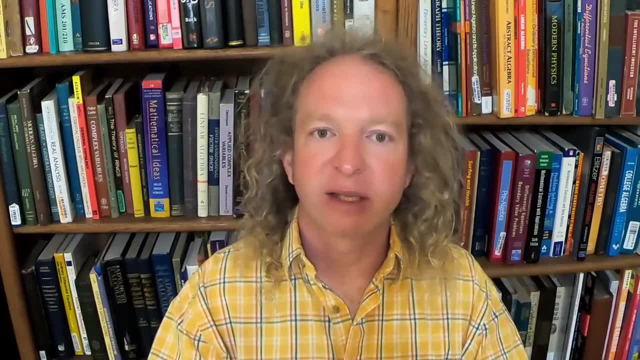 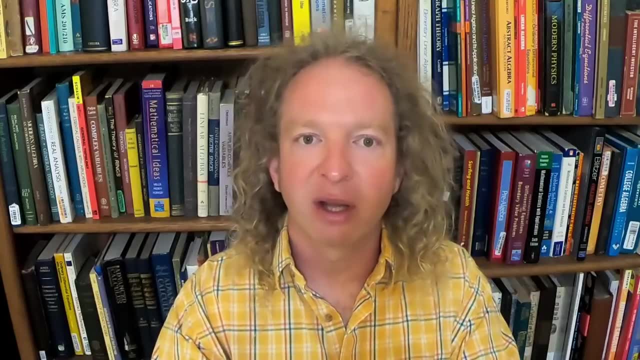 For many people, calculus is one of the hardest math classes that they will ever take in their entire lives. Most of us take math in high school and then some math in college, And many people actually stop with calculus. Calculus is it. Therefore, it's the hardest math class. 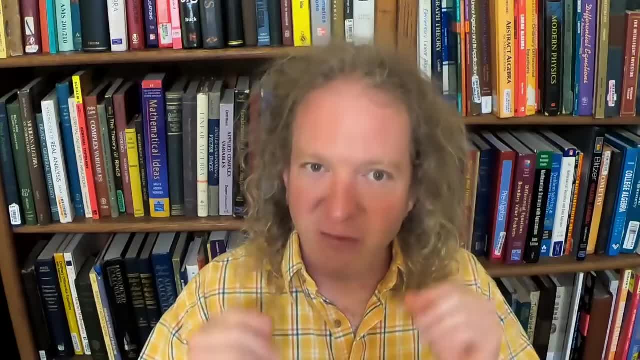 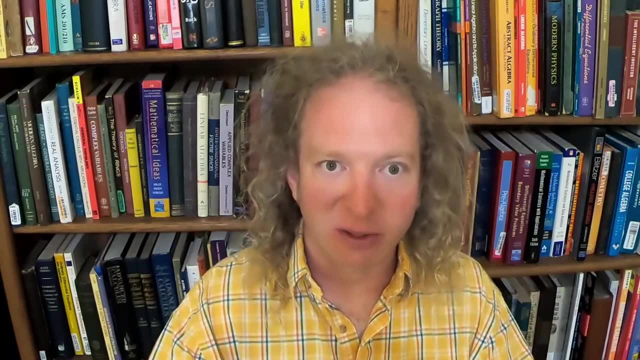 that they ever take. In this video, I'm going to share several things that you can do if you're taking calculus that will help you get an A in the class. The first thing that you should do if you're taking calculus is to actually do the homework. It is absolutely. 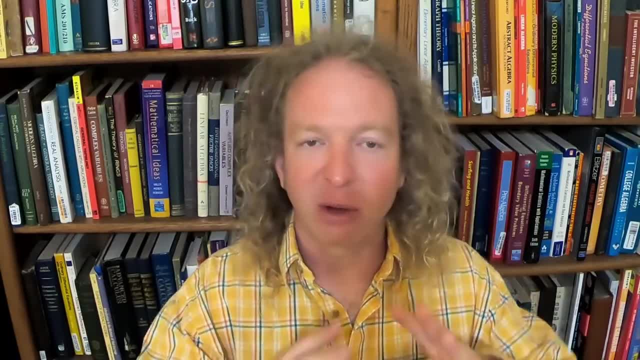 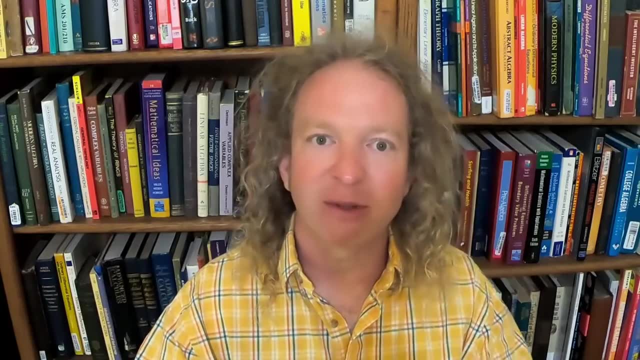 critical that you do all of the homework. I mean, don't skip any problems. If there's like 30 problems in each section or 20 problems in each section, it doesn't matter how many problems are assigned, You should do all of them. This is an absolute requirement, And 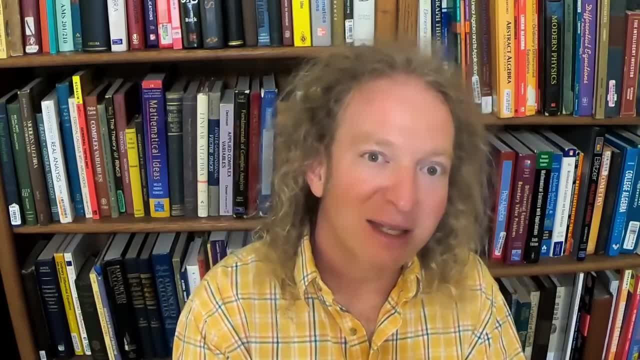 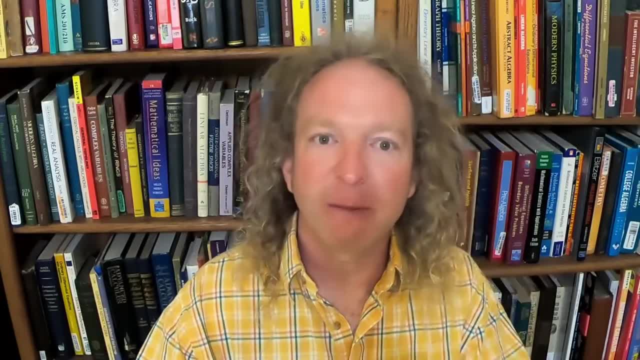